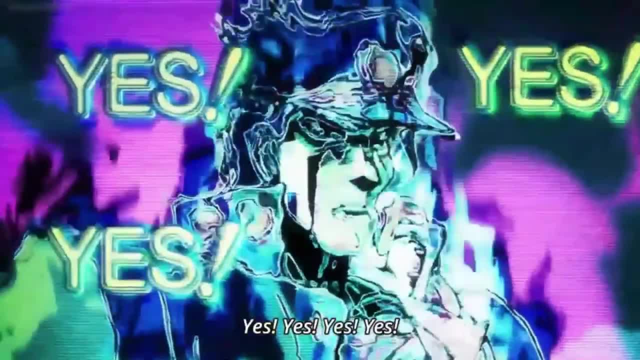 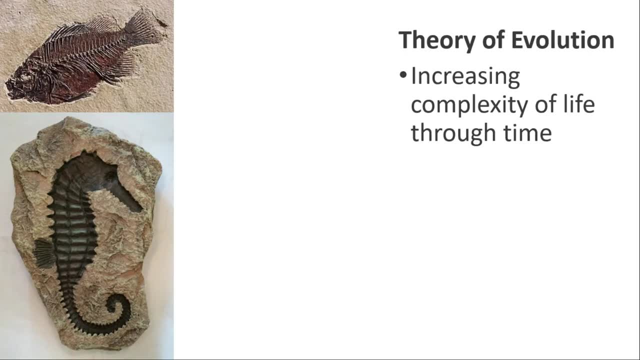 Right, Remember the rock cycle. Now preserved in rocks are fossils, or the remains and traces of plants and animals that have lived and died throughout the earth's history. The fossil record provides scientists with one of the most compelling evidence for Charles Darwin's theory of evolution. This is about the increasing complexity of life through. 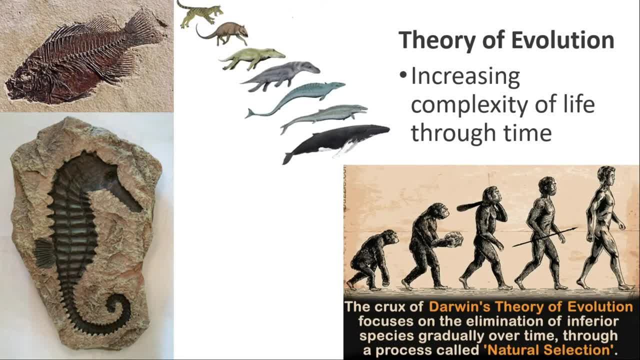 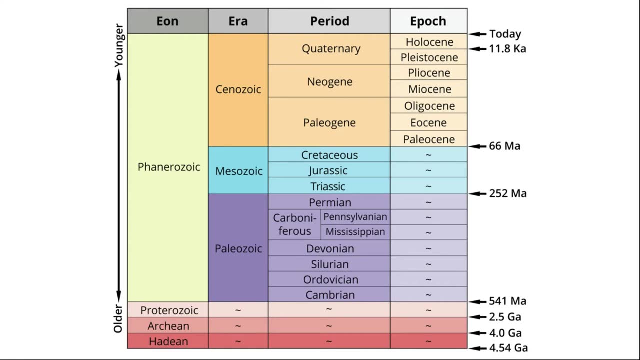 time. So the crux of Darwin's theory of evolution focuses on the elimination of inferior species, gradually over time, through a process called natural selection. Now this figure, the geologic time scale, which is the timeline of the history of the earth. 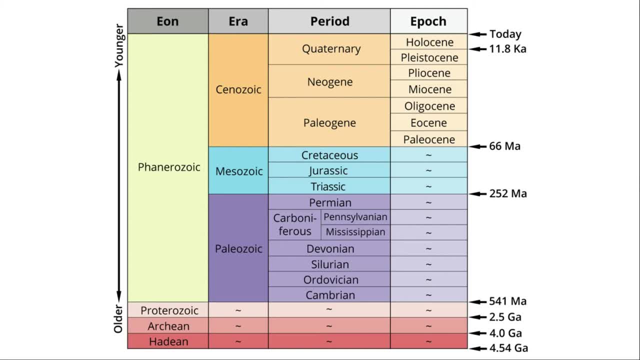 is based on the rock record. Geologic time is divided into hierarchical intervals, the largest being eon, followed by era period and epoch. The subdivision of geologic time is based on significant events in the earth's history as interpreted from the rock record: The mass extinction, which led to extinction of 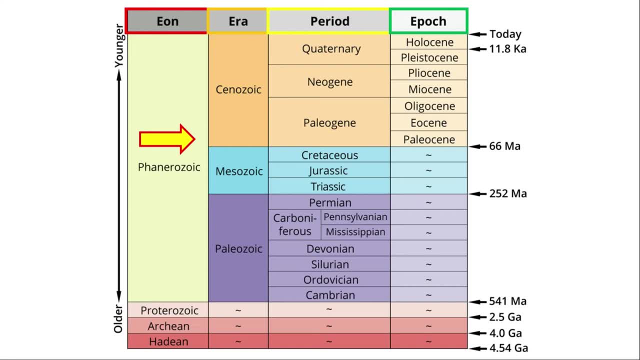 the dinosaurs occurred around 66.4 million years ago. Now remember this mass extinction event may have been pivotal in the race of the dominance of the mammals during the Cenozoic era. Now remember this mass extinction event may have been pivotal in the race of the dominance of the mammals during the Cenozoic era. 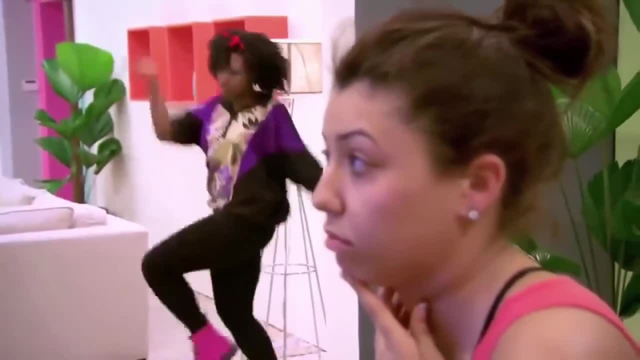 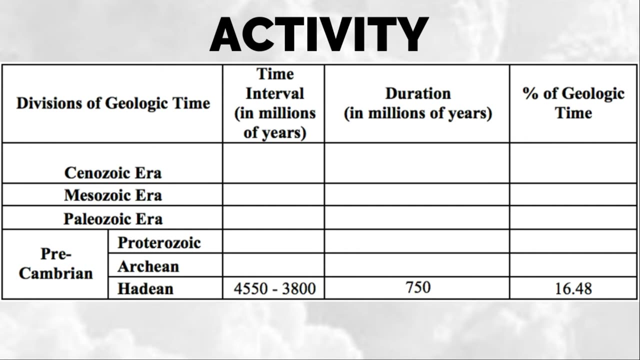 Now let's have an activity. What you need to do is you have to fill this table up. Afterwards, you have to make a pie chart with respect to the geologic time scale provided in the table. are you kidding? Are you kidding me? I'm getting angry. I'll give you 5 minutes to accomplish this. I'll give you five minutes to accomplish this. Ok, So, while we're doing that, we have a table right over here, So let's set up this table. So let's set up this table right over here, Evowym. Are you kidding me? Are you kidding me? Okay, So while we're doing this, we have a table with the object. we need to fill this table up. 感謝 grenater teusa. Are you kidding me? Are you kidding me? 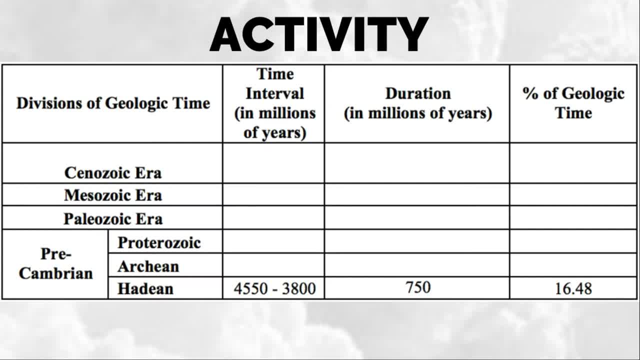 reconciliationiale di Io are doing this, Listen. So one of the first to recognize the correspondence between rocks and time is Nicholas Steno. Steno's principle, namely superposition, original horizontality and lateral continuity, became the foundation of stratigraphy. Again, stratigraphy is the study. 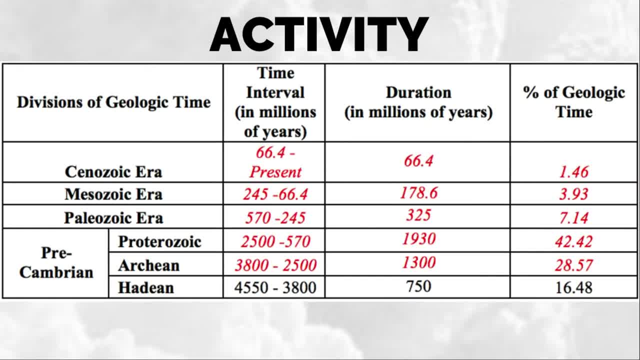 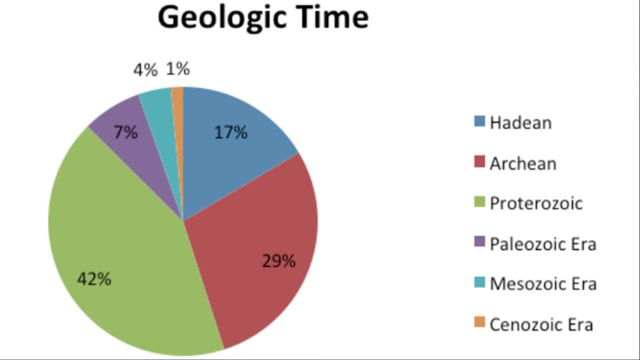 of layered rocks. So this is the correct answer. Okay, so remember, you have to make a pie chart with respect to the geologic time scale provided in the table. Assuming that you have done the pie chart, this figure shows relative proportion of the major subdivisions of geologic time. Now, 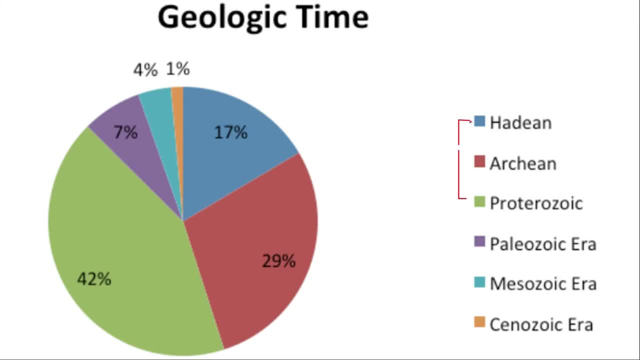 if you notice, the Precambrian, which is the Hadean, Archean and Proterozoic, represents a large part of the geologic time scale. So this figure shows relative proportion of the major of the geologic time, which is about 87%. Yet we know very little of what happened during this. 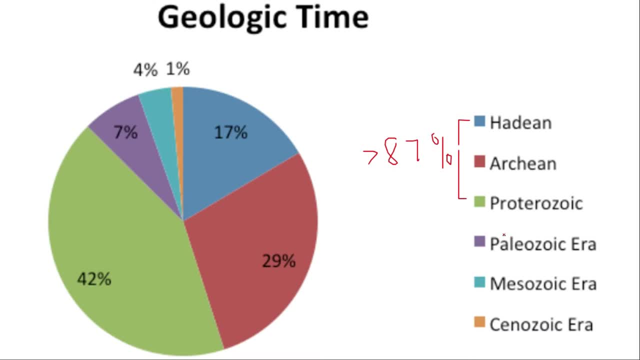 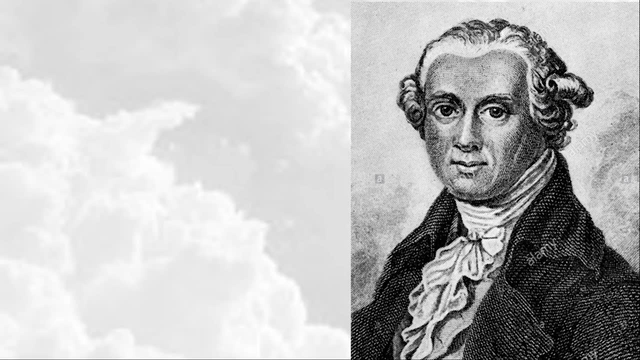 period. Okay, so meaning the record is imperfect or incomplete. One of the earliest attempts to subdivide the rock record into units of time was made by Abraham Gottlob Werner, a German geologist. Werner divided the rock record into the following rock time units: 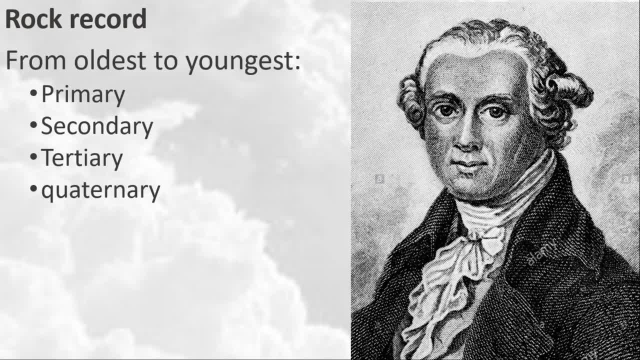 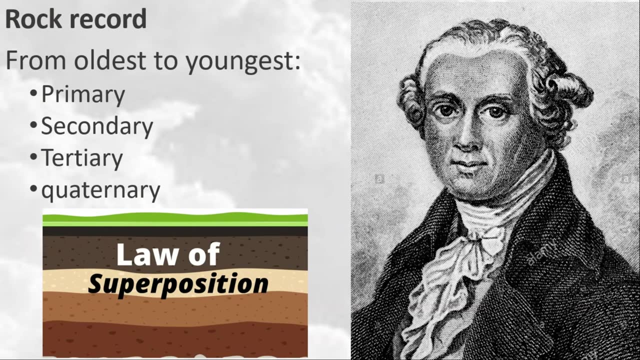 From oldest to youngest. So we have the primary, secondary, tertiary and quaternary. Werner extensively used the law of superposition to establish temporal relationship among the rock units. He states that within a sequence of layers of sedimentary rocks, the oldest layer is at the 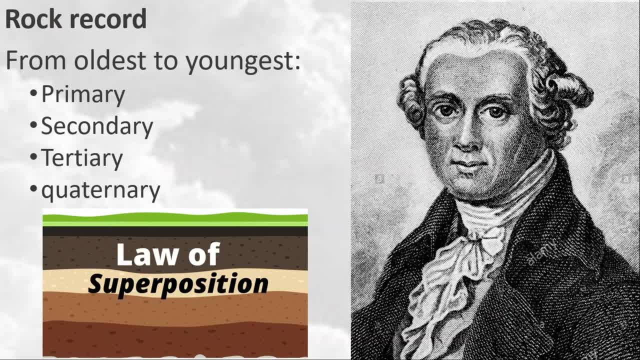 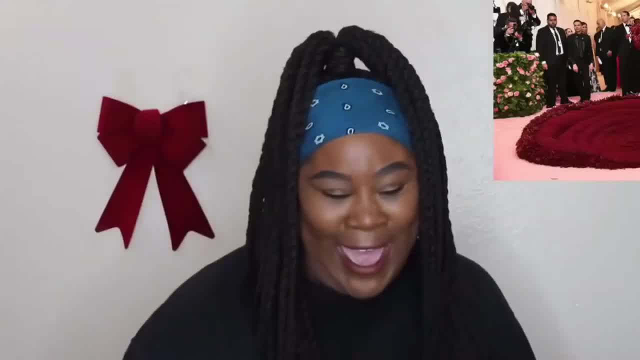 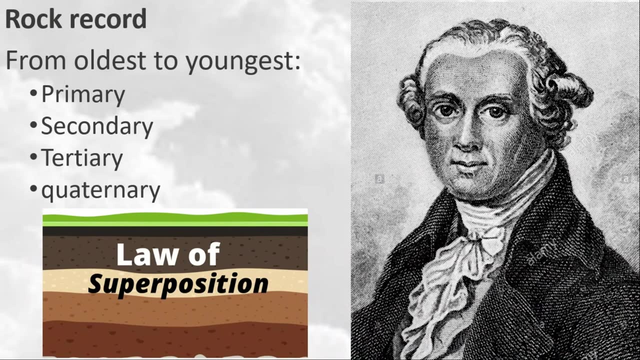 base and layers become younger as it goes up. Okay, so if you remember, you have to make a pie chart to remember our previous discussion about this. Yes, that's it. So I just want you to know that Abraham Werner is also considered to be the father of German geology. 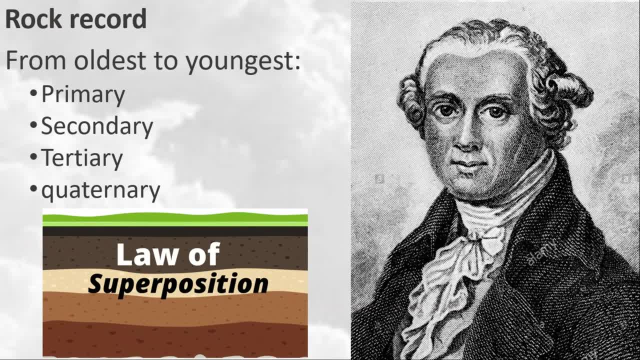 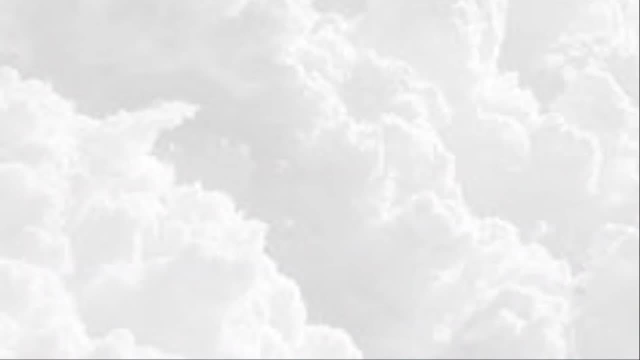 and he is also the proponent of Neptunism, That is, the idea that all of the earth's rocks were formed from an all-encompassing ocean. Fossils are also useful in determining the relative ages of rocks. While working in a coal mine, William Strata Smith observed that each 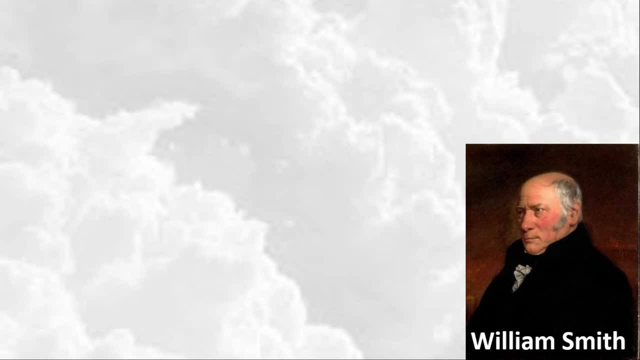 layer or strata of sedimentary rock contains a distinct assemblage of fossils which can be used to establish equivalents between rock units separated by long distances. Moreover, he observed that these fossils succeed each other vertically in a definite order. Okay, so this is the first. 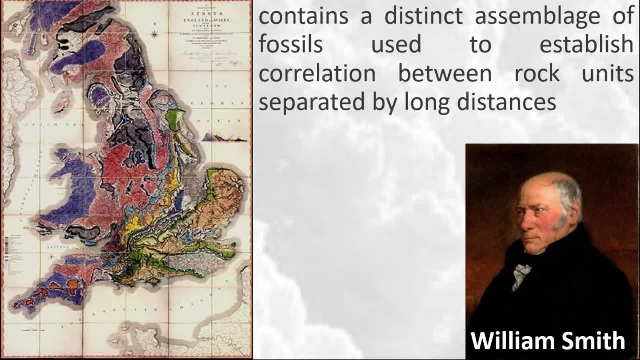 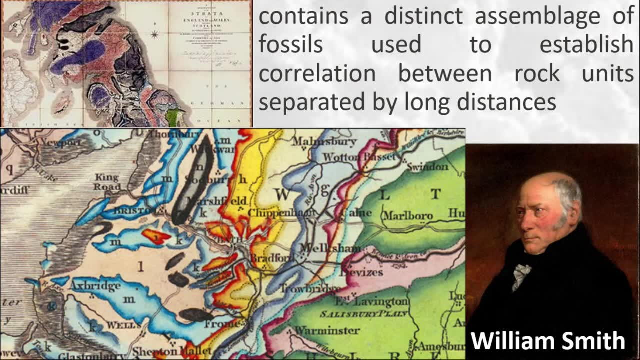 example, This figure shows the geological map of England, Wales and part of Scotland in 1815, and this one is Smeets' 1820 map, called A New Geological Map of England and Wales, which illustrates the complex geology surrounding Bath, England. So these figures are from NASA Earth Observatory. In contrast to William Smith, who primarily used a fossil from the 19th century, this one is from the 19th century. The other two are found in the process of creation, but only when it is completed. This one is called Morel's map, which which is based on a geological map of England and Wales. 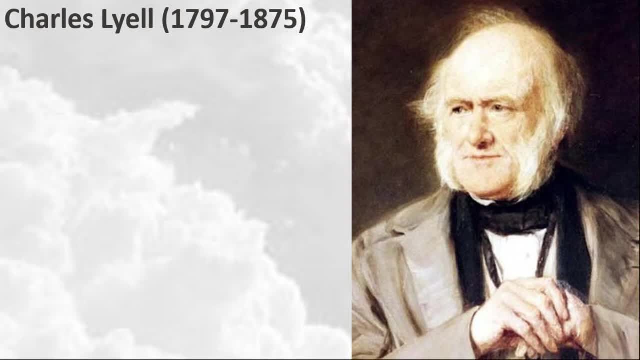 This one is called Morel's map, which which is based on a geological map of England and Wales fossils to identify rock layers. Charles Yell, a British lawyer and geologist, recognized the utility of fossils in subdividing geologic time. on the basis of fossils, He was able to subdivide. 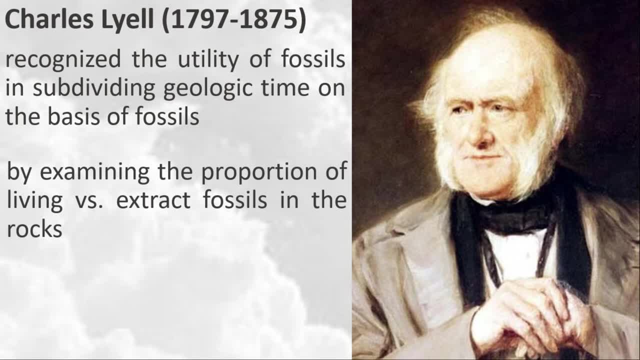 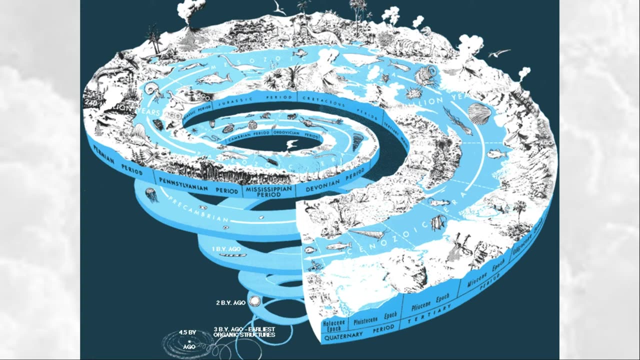 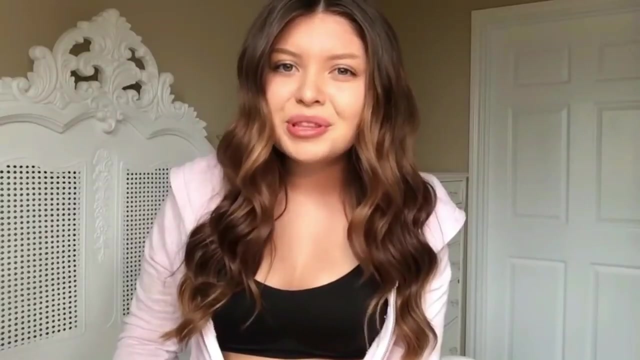 the tertiary by examining the proportion of living versus extinct fossils in the rocks. The bottom line is: fossils are essential in the subdivision of the geologic time, So this figure shows the evolution of life through time. The underlying reason for this definite and orderly succession of fossils in the rock record is, seriously, what the are you doing? Organic evolution. 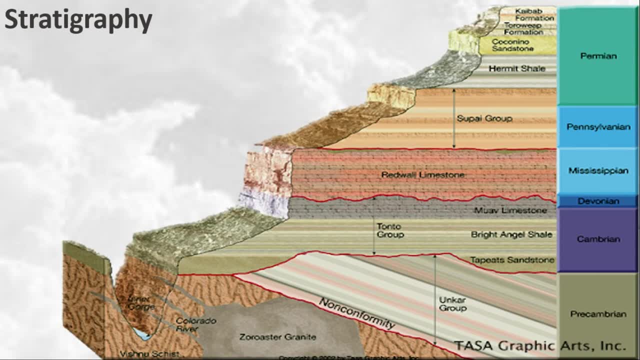 So we have studied stratigraphy, right. As we have said, stratigraphy is a branch of geology concerned with the study of rock layers and layering. It's primarily used in the study of sedimentary and layered filtration. Now, a subdiscipline is what we call biostratigraphy. 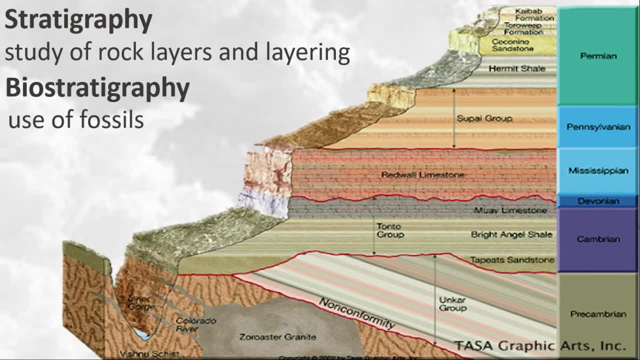 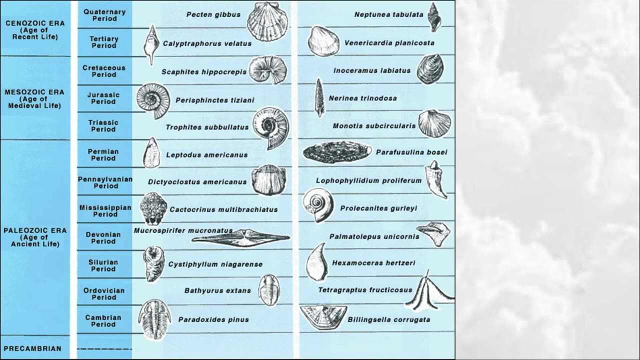 This deals with the use of fossils in the correlation and establishments of the relative ages of rocks. In the next video we're going to study the geologic time scale. okay, It's over, We are screwed. Now we have this thing called index fossils, So this figure